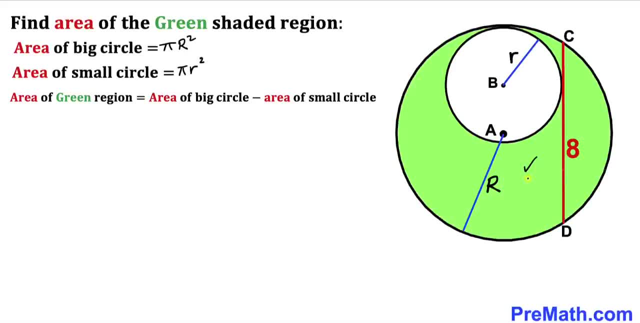 of this green shaded region is going to be equal to the area of this big circle minus the area of this smaller circle, and we already know the area of this big circle and the area of the smaller circle as well. So, therefore, the area of this smaller circle is going to be pi r square, and 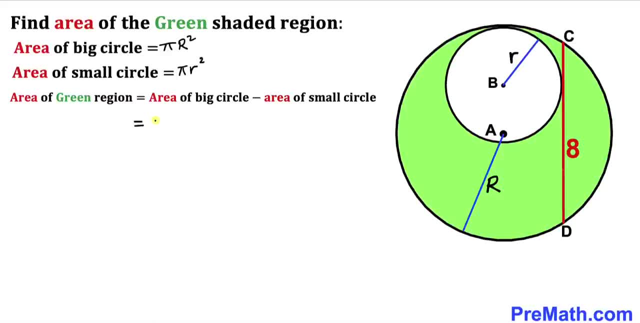 this green shaded region is going to be simply pi r square minus pi lowercase r square, and we can see pi is in common, so I can factor that one out. So we simply got pi times uppercase r square minus lowercase r square, and now our task is to find the value of this smaller circle. So let's go. 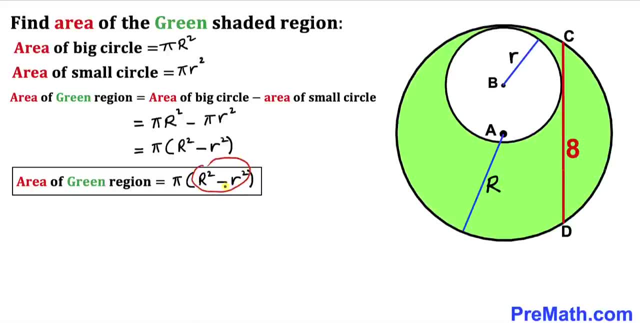 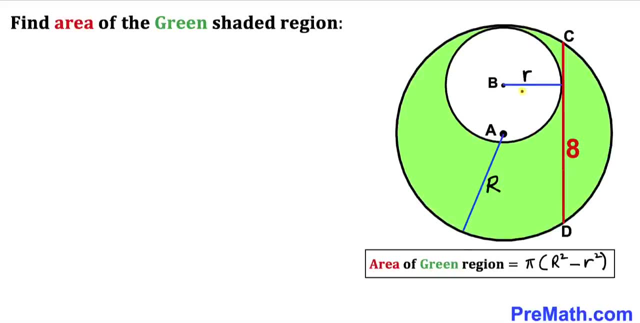 ahead and take a look at our next step. Let's focus on this radius of this smaller circle. and now let's recall the circle theorem. According to this theorem, the angle between the radius and the tangent line will always be 90 degrees, as you can see in this diagram. So therefore, 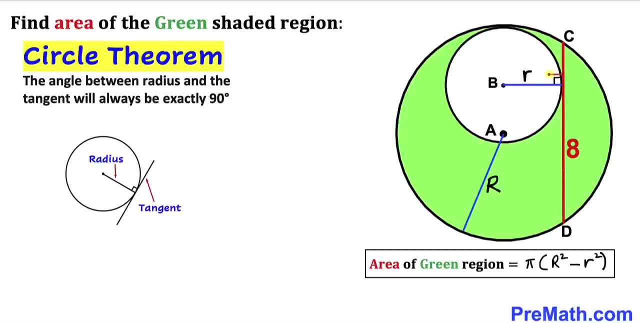 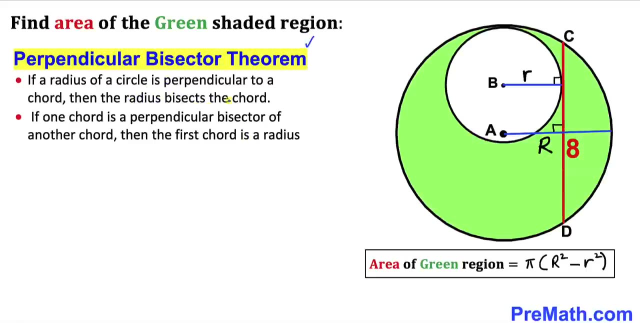 in our case, this angle between this tangent and the radius is going to be 90 degrees as well. And now let's focus on the radius of this larger circle. and now let's recall the perpendicular bisector theorem. According to this theorem, if the radius of a circle is perpendicular to a chord, 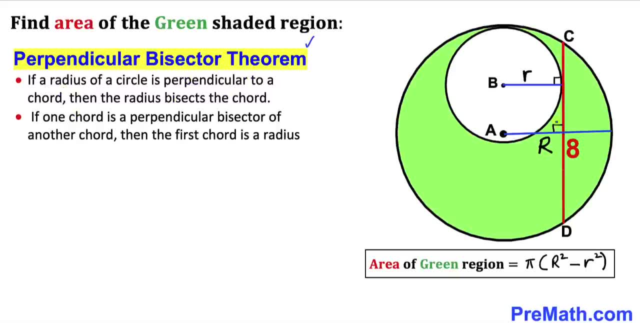 then the radius bisects the chord, As we can see that this radius is perpendicular to this chord. so therefore this radius is going to bisect this chord. cd into two equal parts. The total length is eight, so therefore this side length is going to be half of that one. 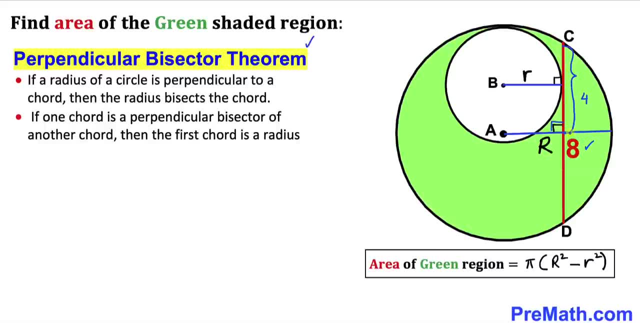 that is going to be four units, and likewise this length is going to be four units as well. So therefore, our this distance ce turns out to be four units. and now we can see that these two line segments are perpendicular to this chord cd. So therefore, this length is going to be equal to this. 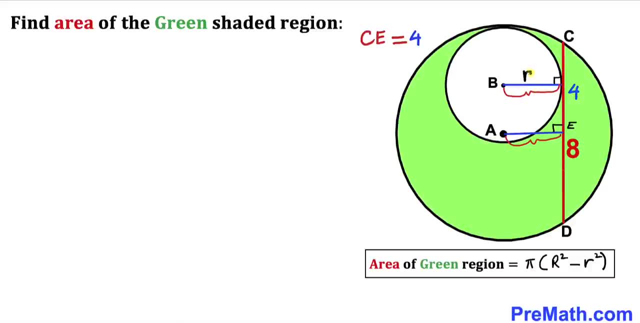 length. If the length of this one is lowercase r, so this is going to be lowercase r as well. So therefore, this line, segment AE, equals to r. and here's our next step. Let's go ahead and connect these two points, A and C. Let me go ahead and draw a straight line, and here's our much nicer 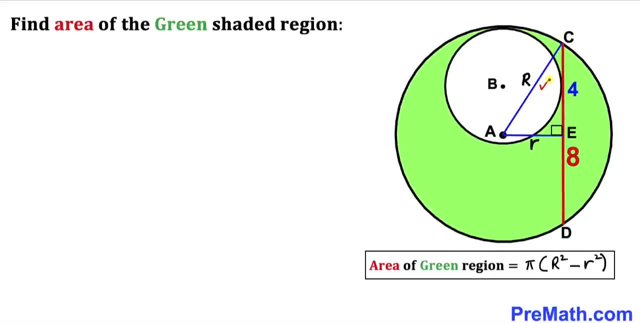 looking diagram and we can see that this AC is the radius of this larger circle and this is represented by uppercase R. And now let's focus on this triangle. We call this triangle aec and we know that this is a right triangle, So therefore we are going to use the 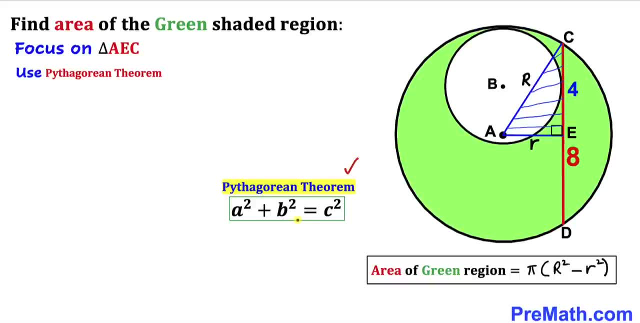 Pythagorean theorem. and here's the Pythagorean theorem: a square plus b square equal to c square. Let me go ahead and call this longest leg our side c. I'm going to call this leg a and this side b. So let's go ahead and fill in the blanks. In our case, a is r, b is 4.. 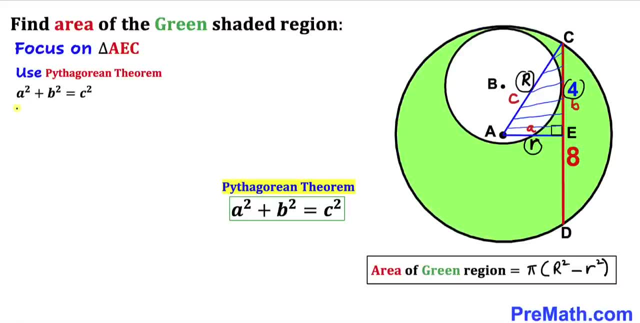 and C is uppercase R. Let's go ahead and fill in the blanks. So this is going to be R square plus 4 square equal to uppercase R square. Now let's go ahead and simplify. So we got R square plus 4 square is 16 equals to uppercase R square. Let's go ahead and move this. 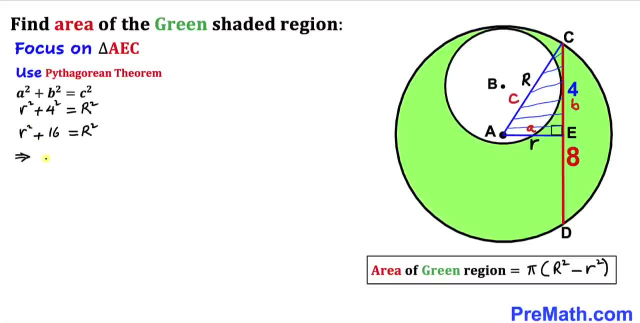 lowercase R square on the other side. So therefore we are going to get uppercase R square minus the lowercase R square turns out to be equal to 16.. And now let's recall from our previous step: the area of this green shaded region equals to pi times.